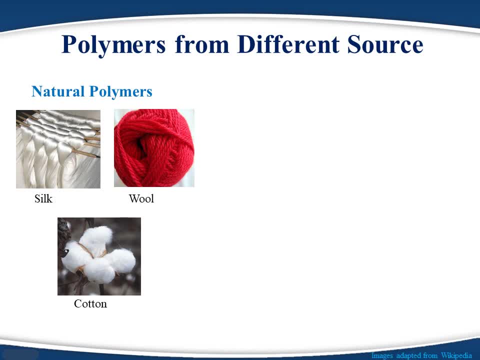 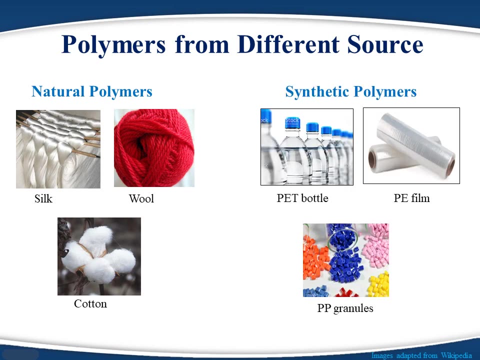 availability. Also, natural polymers cannot be melted and molded into different shape. Discovery of chemical method to make man-made polymers, which are also called synthetic polymers, was a pivotal point in this amazing success story, As synthetic polymers can be industrially. 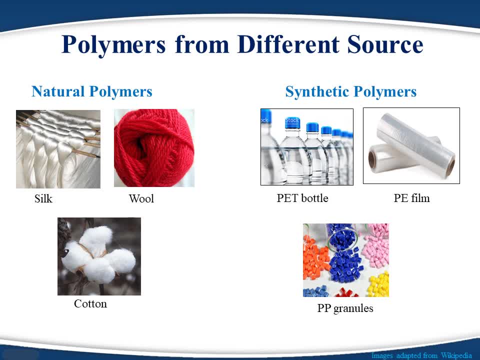 produced at large and can be used for many different purposes. the process of making polymers at large scale. it led to significant reduction in the cost of polymer. Nowadays, synthetic polymers are blended with natural polymers to achieve similar comfort at lower cost. 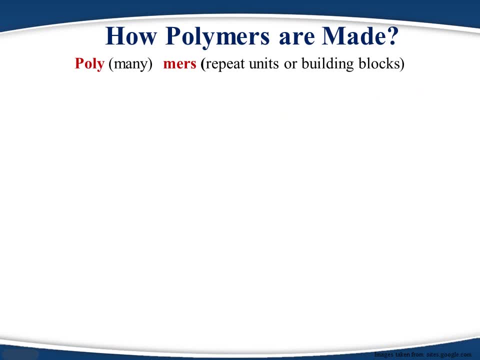 Now the question is how polymers are formed, both in nature and in an industrial reactor. In a very basic sense, polymers are made or formed by joining small molecules in a single chain. These small molecules are called monomers. The process of making polymers from monomer. 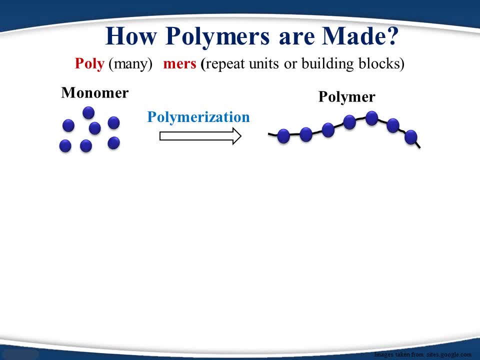 is called polymerization Based on reaction kinetics. polymerization reaction can be classified into addition polymerization and condensation polymerization. In addition, polymerization polymers are formed in three steps. In initiation step, a small number of monomers reacts with initiator molecules to form active monomer or free radical. 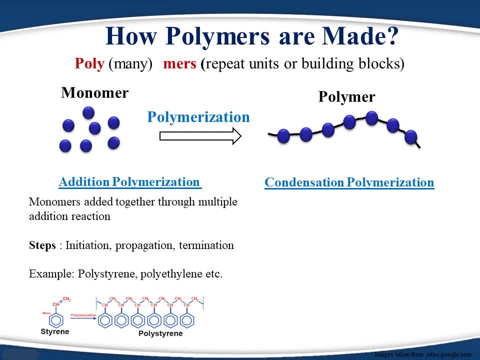 In propagation step, the active monomer reacts with a large number of monomers through radical transfer and forms a long chain. And finally, in termination step, two active chains react with each other to form a neutral polymer chain. In condensation, polymerization monomers. 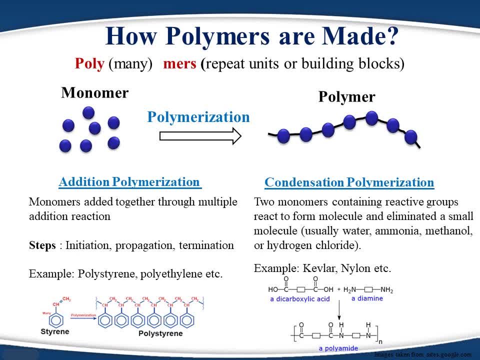 are formed by joining a small number of monomers. Polymers contain functional groups, like acidic and basic groups, which, under appropriate conditions, react with each other and form covalent bonds between them. As the reaction progresses, monomer forms dimer, trimer, tetramer and so on. Eventually, sufficient monomer reacts. 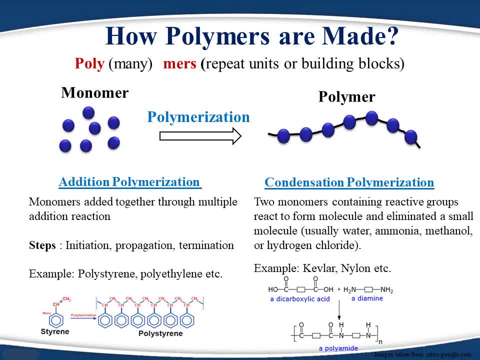 to form polymer chain. In a very general sense, we can say that a monomer which contains a double bond can be polymerized by addition polymerization and a monomer which contains functional group can be polymerized using condensation polymerization. For more detail about the reaction mechanism and merit and demerit of each mechanism, please. 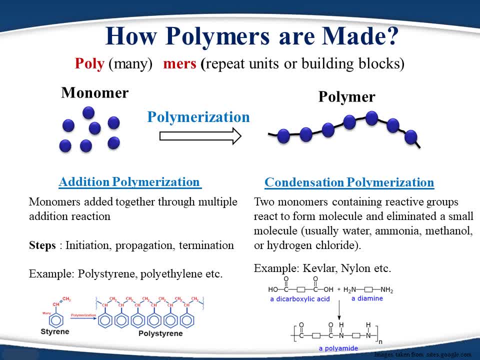 watch our video on polymer synthesis. Anyways, during polymerization, reaction condition can be selected to achieve polymers. Polymers can be used to create different types of monomers. Polymers can be used to create different types of monomers. 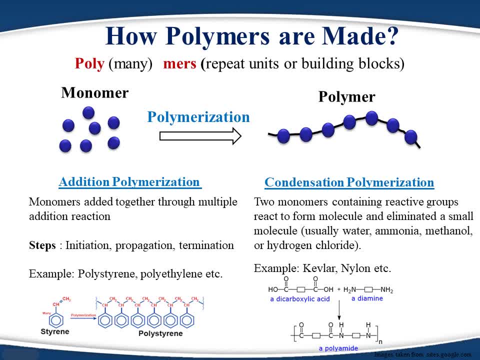 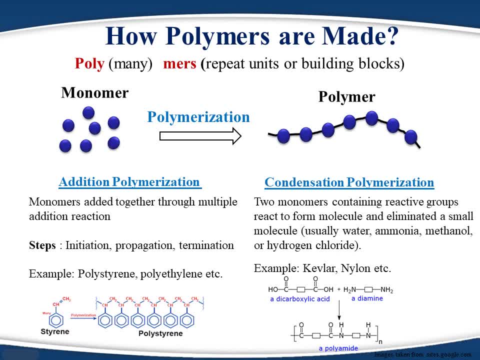 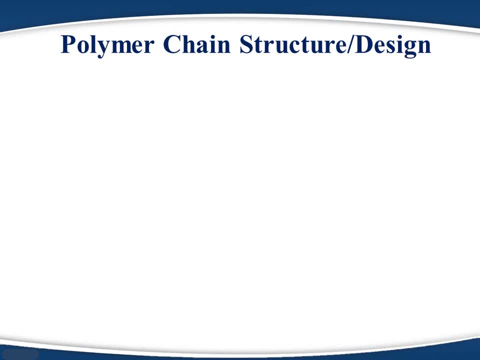 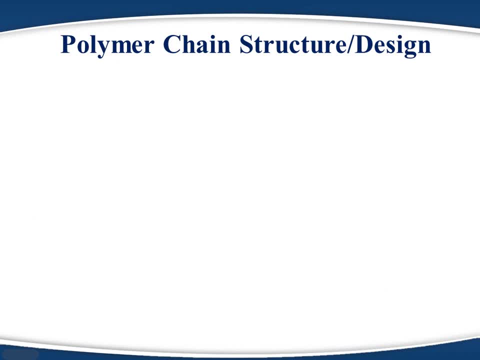 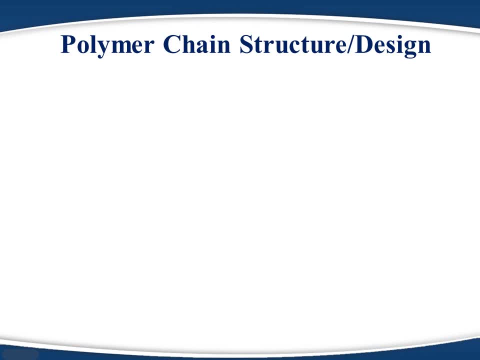 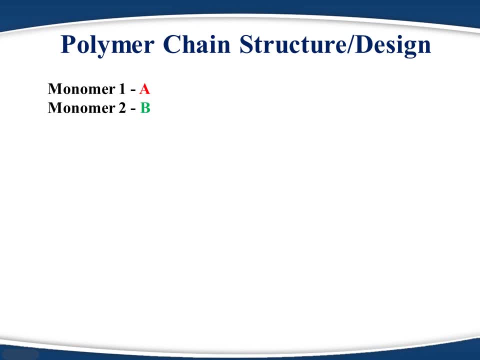 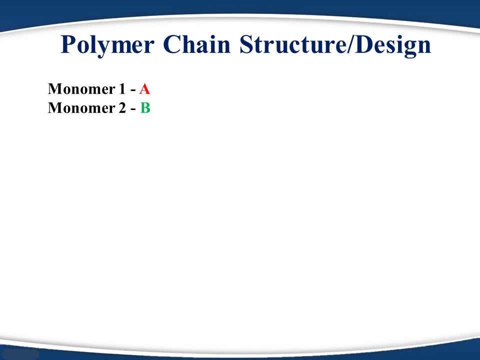 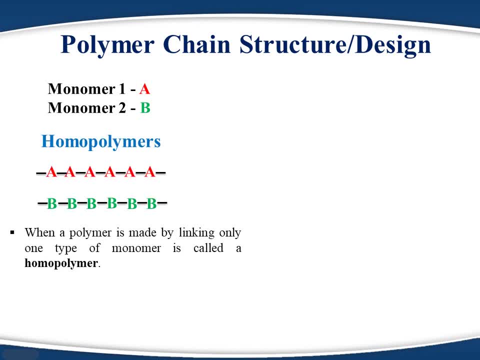 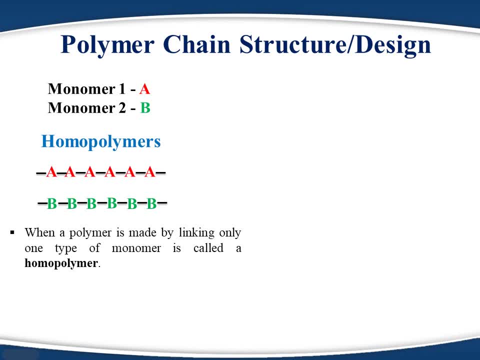 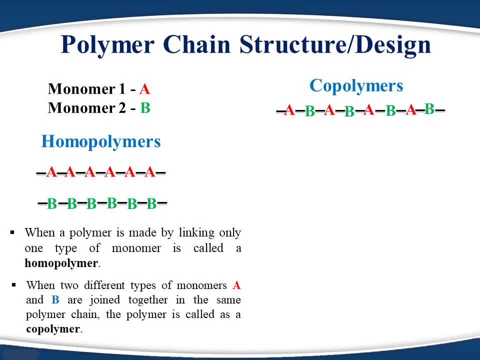 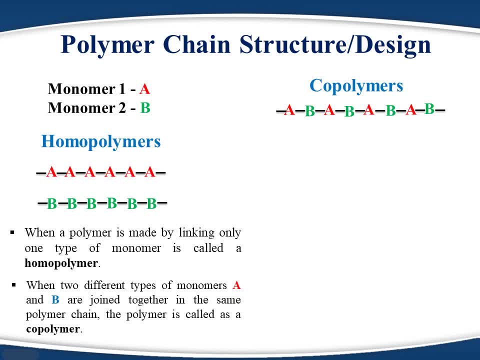 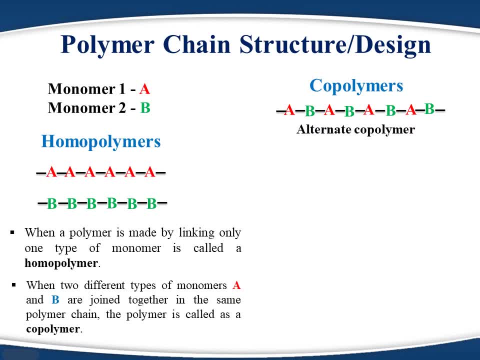 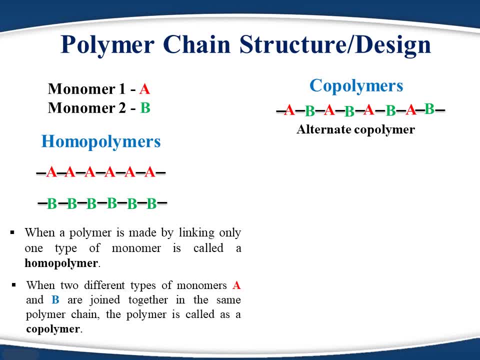 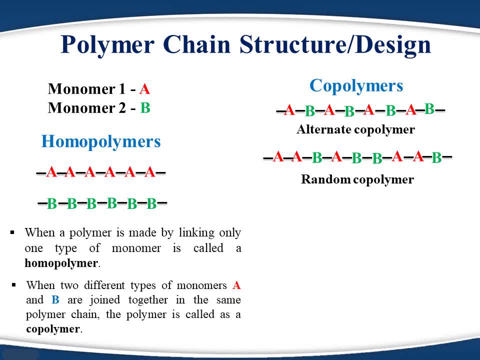 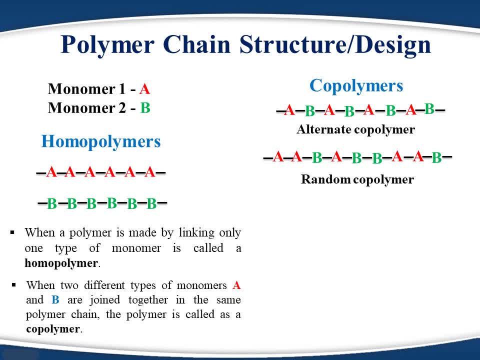 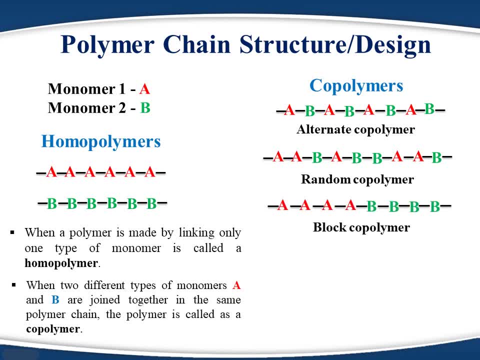 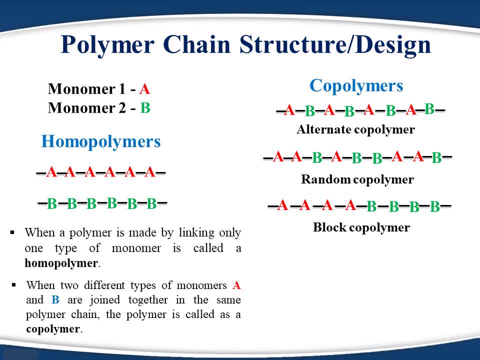 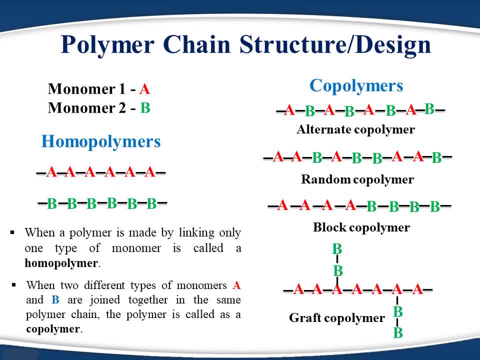 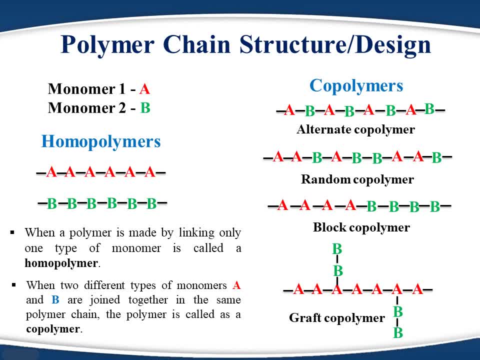 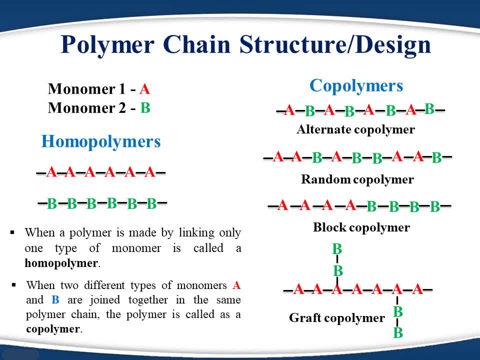 properties of polymer strongly depends on the monomer type. let's assume monomer a is a bulky monomer which form a strong polymer with limited flexibility, whereas monomer b is a small monomer and form polymer with excellent flexibility but poor strength. so if we want to have a material, 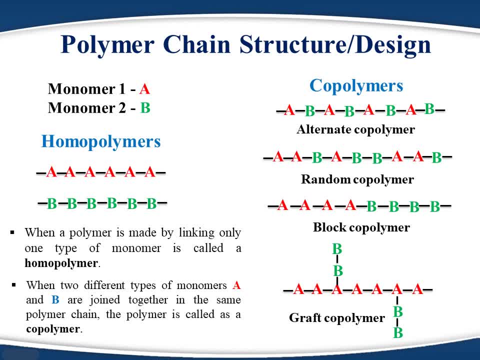 with good flexibility and strength then we can design a polymer chain containing both a and b monomers. but we have to be careful because if the size of a and b monomers are significantly different, we may lose the properties of both monomers in order to keep properties of both. 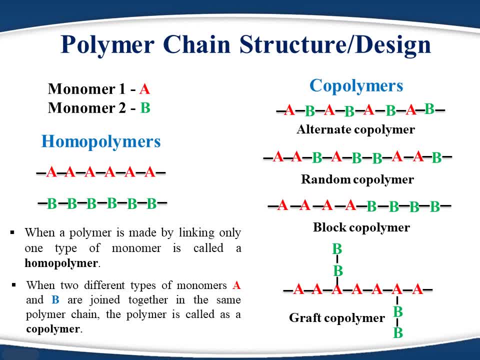 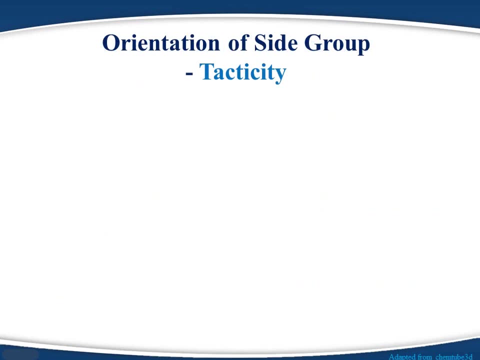 monomers. we can design polymer chain containing blocks of a and b monomers. in industry, block length are precisely controlled to develop polymer with very specific properties. properties of polymer also depends on orientation of side group. in the picture we can see that side group of polystyrene polymer are oriented on one side of main chain if side group of a polymer are. 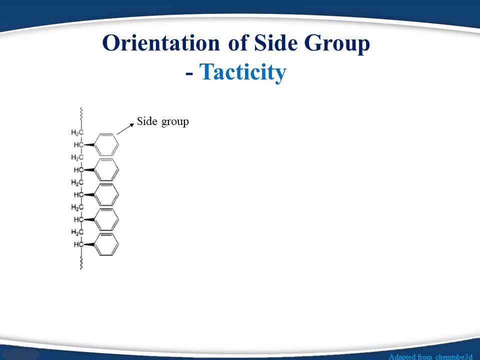 oriented on one side of the main chain, it is called ionized polymer, polymer, polymer polymer polymer, isotactic polymer. if the side groups are oriented in an alternating sequence, polymer is called syndiotactic polymer, and if side groups are randomly oriented, they are called a tactic polymers. based on the structure, we can say that isotactic and syndiotactic polymer chains are. 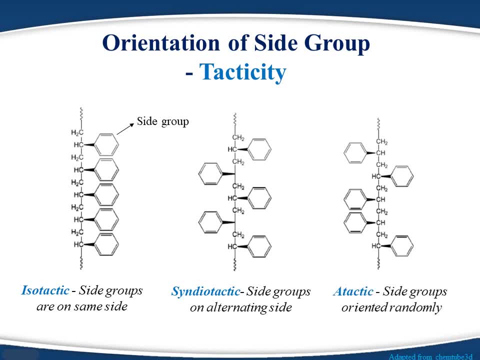 symmetric. therefore, two isotactic or two syndiotactic polymer chains can come in close proximity and can form an ordered structure. close proximity can also enhances the intermolecular interaction force. as a result, isotactic and syndiotactic polymers are usually very strong. as a tactic polymer chains are asymmetric. two a tactic polymer chains cannot come in. 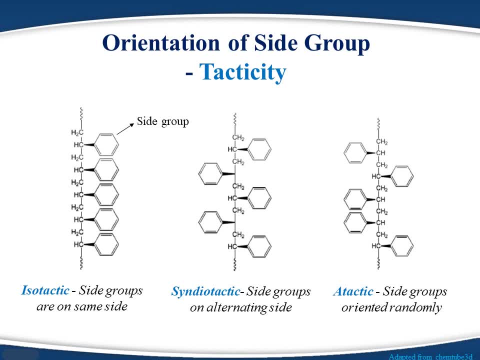 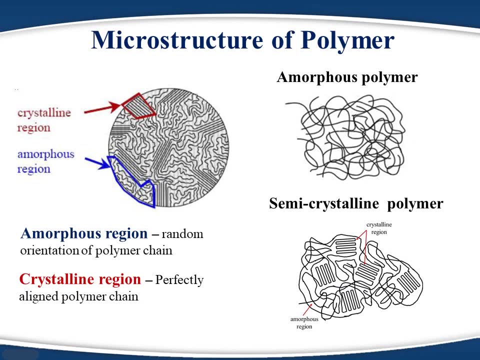 close proximity, therefore a tactic. polymers are usually weak, but they very high flexibility. Two types of microstructure are usually observed in polymer, namely amorphous and crystalline. In amorphous region, polymeric chains are randomly oriented, whereas in crystalline region polymer 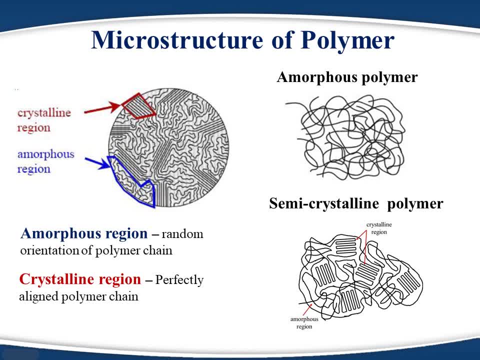 chains form highly ordered structure. As I have previously mentioned, isotactic and syndiotactic polymer chains can pack very well, so they form crystalline polymer, whereas atactic polymer chains cannot pack, so they always form amorphous polymer. Typically, strength of polymer depends on the percentage crystallinity and flexibility depends. 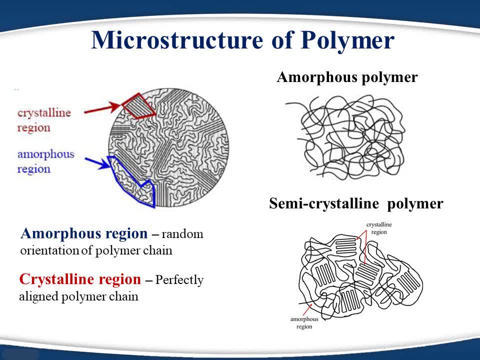 on amorphous content, A trivia: why a polymer can be 100% amorphous but not 100% crystalline? The answer is: end of polymer chain is physically and chemically very different than main chain. So chain ends cannot be a part of crystalline region which prohibit polymers to achieve.